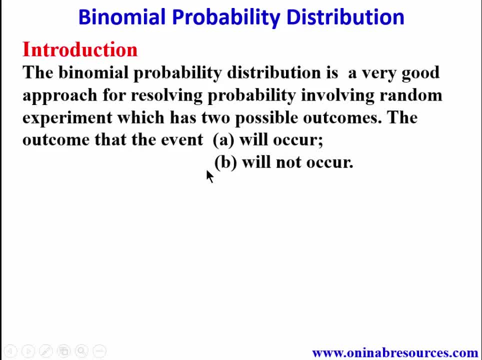 outcomes: the outcome that the event will occur and the outcome that the event will not occur. the tossing of a fair coin and throwing of unbiased die repeatedly are typical examples. in the case of a coin, we consider it either a head or not a head. it could be. 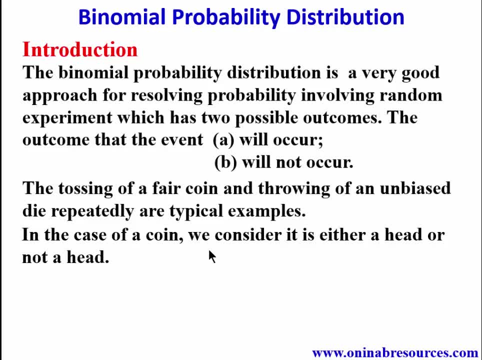 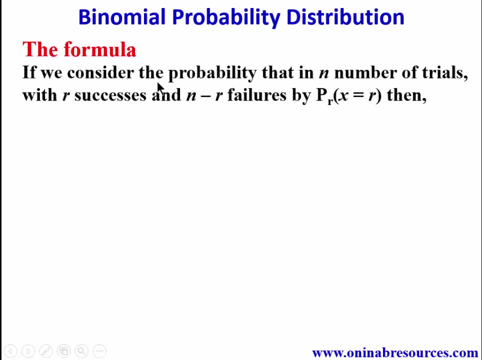 either a tail or not a tail, and invariably there are two options there. if it is not a head, then it is a tail. also for a die. we may consider the event of having six or not six and any other choice of numbers. now. we now look at the formula. if we consider the probability that in n number of trials 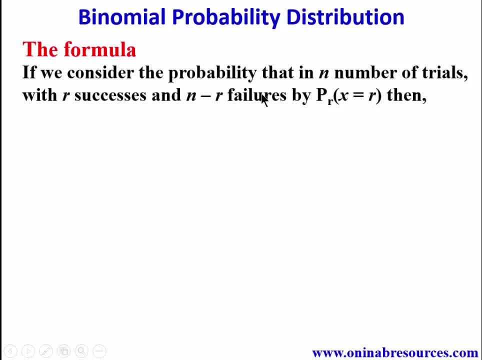 with r subtraction, the probability of success is an n minus r. failures by probability of x is equal to r. then probability of x is equal to r will be: n combination r, p raised to power r, q raised to power, n minus r, where p is probability of success and q is the probability of failure. recall: n combination r. 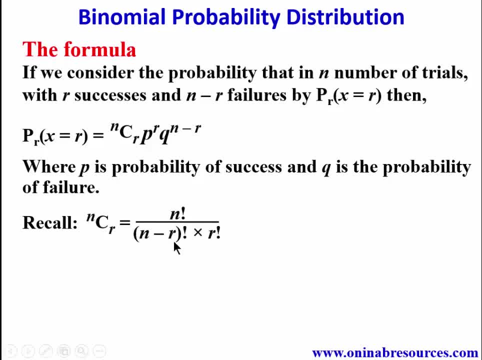 is n factorial. over n minus r factorial. times r factorial. also note that the events are independent of one another for the number of trials. remember: if is a die, you threw the first one. the outcome will not affect the truing of the second one. repeatedly in that order, the same thing. 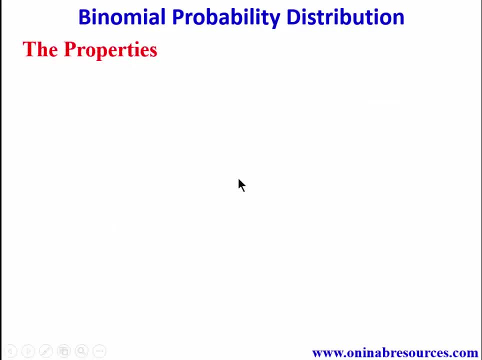 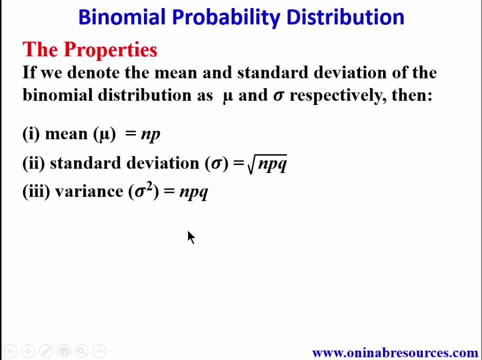 a die. now we look at properties of binomial probability distribution. if we denote the mean and standard deviation of the binomial distribution as mu and Sigma respectively, then the mean mu is NP standard deviation. now, Sigma is equal to square root of NP Q. finally, variance which is Sigma squared is NP Q. so now we 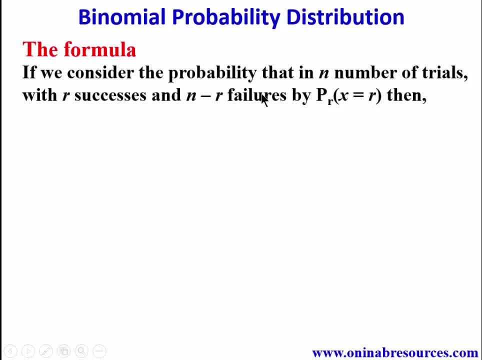 with r subtraction, the probability of success is an n minus r. failures by probability of x is equal to r. then probability of x is equal to r will be: n combination r, p raised to power r, q raised to power, n minus r, where p is probability of success and q is the probability of failure. recall: n combination r. 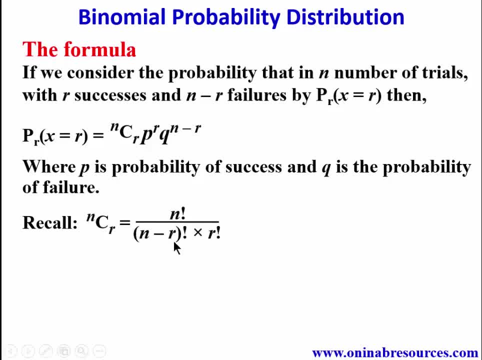 is n factorial over n minus r factorial. times r factorial. also note that the events are independent of one another for the number of trials. remember: if it is die, you threw the first one. the outcome will not affect the trying of the second one. repeatedly in that order. the same thing for dobre. 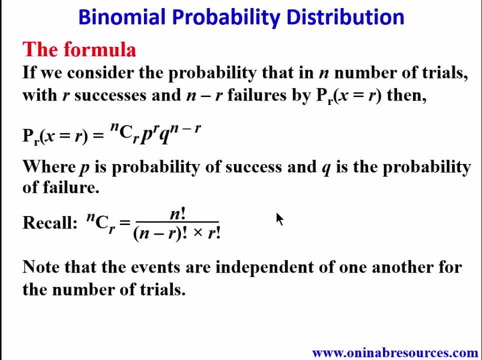 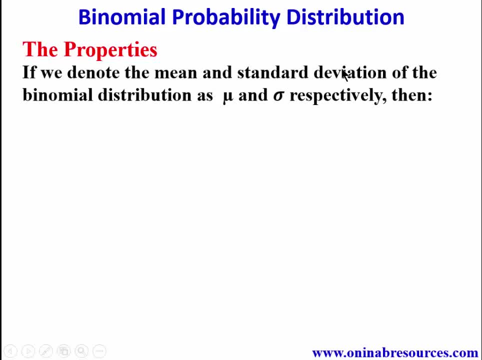 the final results of theggatively faltw is equal to the number of trials. wi visitingcümi outcom of a die. now we look at properties of binomial probability distribution. if we denote the mean and standard deviation of the binomial distribution as mu and sigma respectively, then 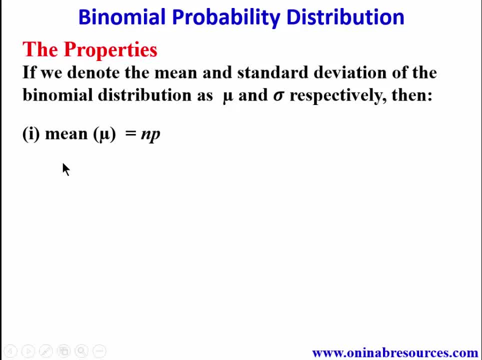 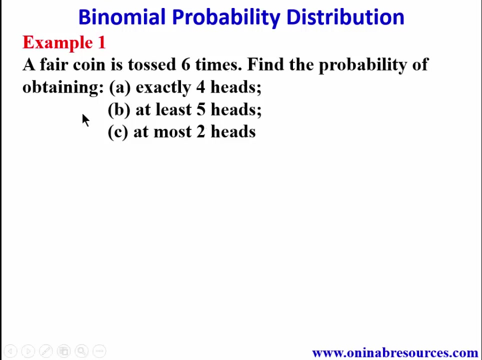 the mean mu is np. standard deviation, that sigma is equal to square root of npq. finally, variance which is sigma squared is npq. so now we go into solving problems. example one: a fair coin is tossed six times. find the probability of obtaining a- exactly four heads, b- at least five heads, and c. 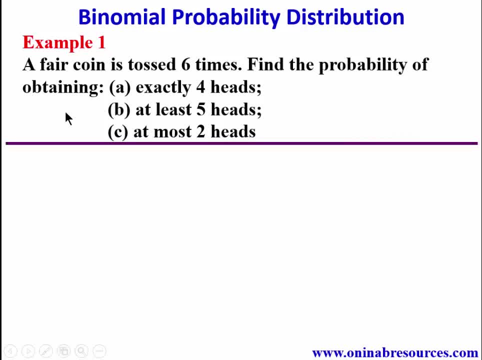 at most two heads. so in our solution we bring in the binomial probability distribution formula, that is, we need to get our r, our n, our p and our q. so also we get our n. so here the probability of success here is 1 over 2, and also the probability of failure. 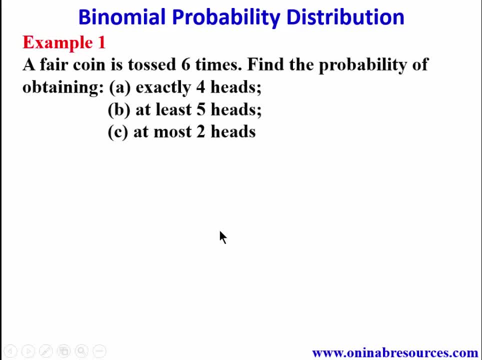 go into solving problems. example one: if a coin is tossed six times, find the probability of obtaining a exactly four heads be at least five heads and see at most two heads. so in our solution we bring in the solution, we bring in the solution, we bring in the. 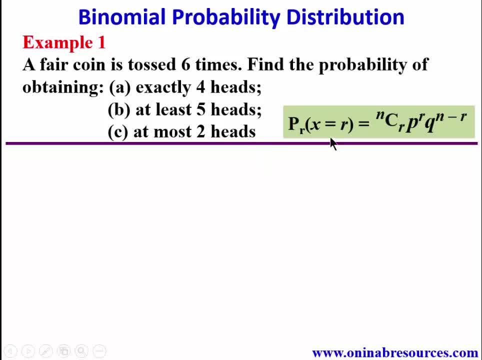 binomial probability distribution formula. that is, we need to get our, our n, our P and our Q, so also we get our n. so here the probability of success here is one over two and also the probability of failure, that is, probability of not getting head, is one over two. 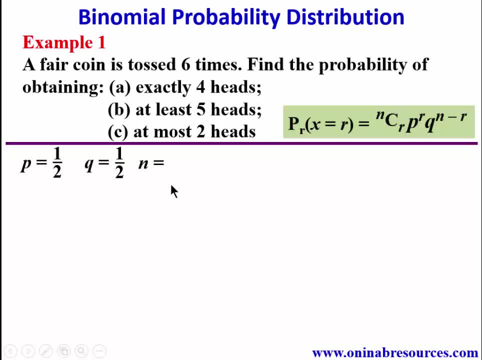 if the, so our N is equal to E. if the is one over two, then we'll look at our N. the number of times the coin is tossed is our n. so we have it R 6 and remember, for our R is 4. so probability of getting exactly four heads out of tossing the coin for six times and that 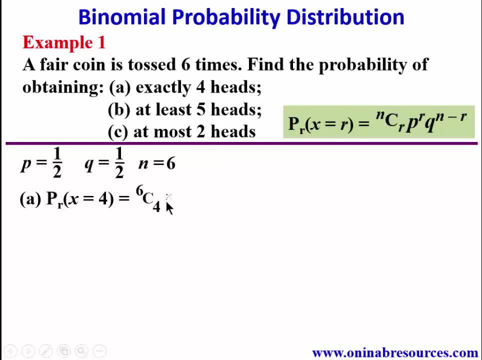 is going to give us six combination of four times success, which is one over two, raised to power r, and our r is four, that's going to be one over two to the power of four. then times failure, which is also one over two, that is not having head. then raised to power n minus r, six minus four, which gives two. so simplifying this. 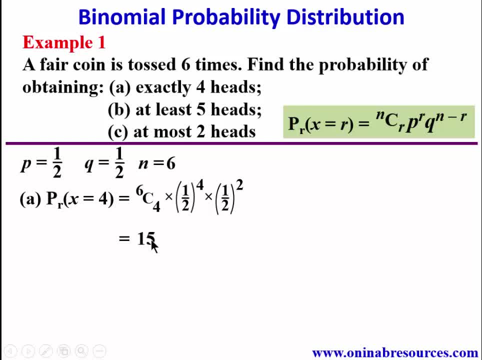 six. combination four is fifteen times one over sixteen times one over four. so here we now have it as fifteen over sixty four, and that is the probability of obtaining exactly four heads. b, the probability of obtaining at least five heads. now, since the probability says at least five heads, so the least you can get out of the six, true, 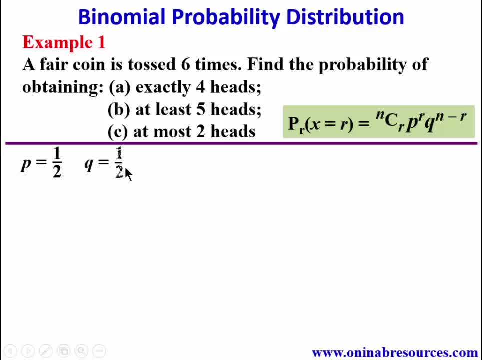 that is, probability of not getting head is 1 over 2. then we look at our m. the number of times the coin is tossed is our n, so we have it as six. and remember, for a our r is four. so probability of getting exactly four heads out of tossing the coin for six times and that is going to give us 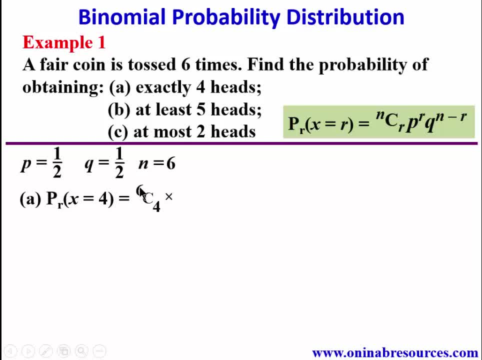 six combination four, times success, which is one over two, raised to power r, and our r is four, that is going to be one over two, to the power of four. then times failure, which is also one over two, that is not having head. then raised to power n minus r, six minus four, which gives two. so simplifying this six combination four is fifteen. 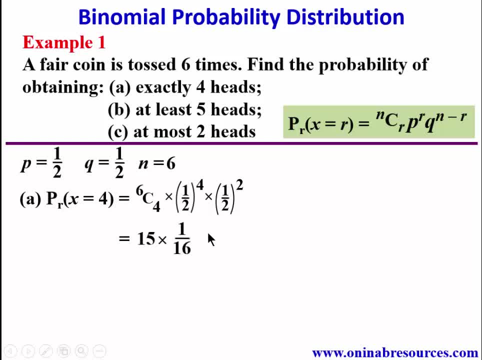 times one over sixteen times one over four. so here we now have it as fifteen over sixty four, and that is the probability of obtaining exactly four heads. b, the probability of obtaining at least five heads. now, since the probability says at least five heads, so the least you can get out of the 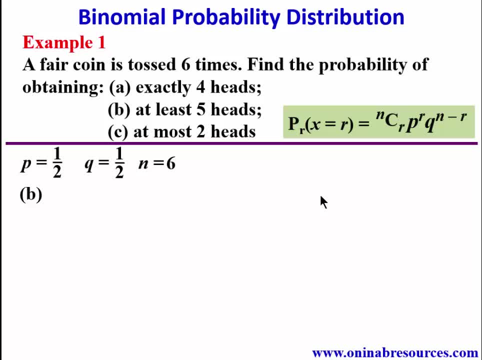 sixth, true is five, so we can have five heads and one tail, or all of them six. so it means it's going to be probability of x is greater than or equal to five, which is going to give us probability of x is equal to five or probability of x is equal to six. and you remember our all means addition. 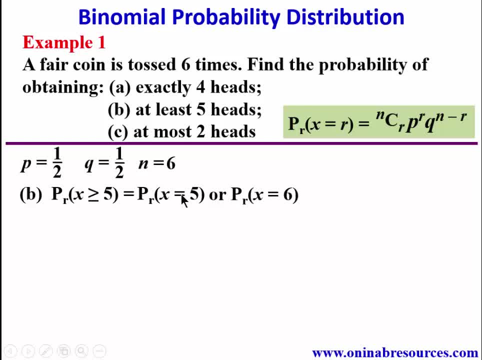 so we then go ahead to find the probability of x equal to five and add it to the probability of x equal to six, so that we now have it as six combination five times probability of success, that is, one over two raised to power five times one over two raised to power one. then this is all. 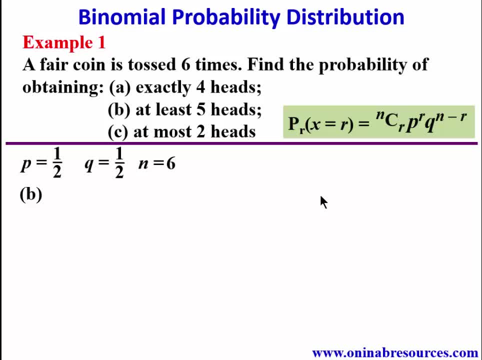 is five, so we can have five heads and one tail, or all of them six. so it means it's going to be probability of x is greater than or equal to five, which is going to give us probability of x is equal to five or probability of x is equal to six, and you remember, 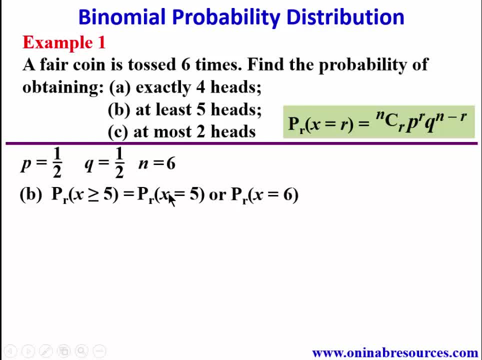 the probability of x is greater than or equal to five. and you remember, the probability of x is equal to five and adding to the probability of x equal to six, so that we now have it as six combination five times probability of success, that is, one over two, raised to power five times one over two. 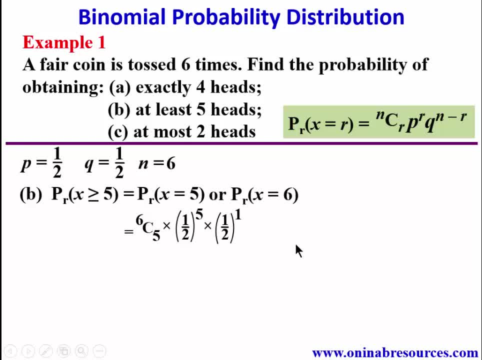 raised to power one, then this is all which means plus for probability of x is equal to six. we have it at six combination: six times p, which is one over two, raised to power six, then times failure, which is one over six raised to power zero. so six combination five gives six times one over thirty, two times one over two. 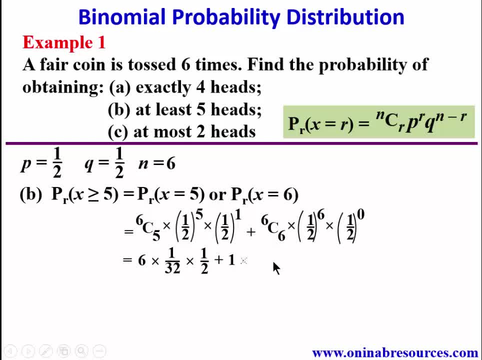 combination 6 is 1 times 1 over 64 times 1, since half raised to power 0 is 1. so, simplifying this, we have it as 6 over 64 plus 1 over 64, and that gives our final answer as 7 over 64, which is the probability of obtaining at least 5. 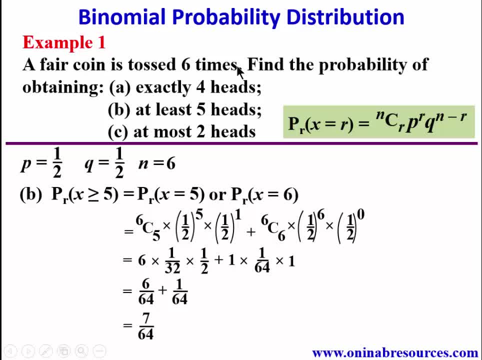 heads when the coin is tossed 6 times. so we go to see part of the problem for seeing at most two, at most the highest, we can get the two heads. so in this case now we are going to have it as P of X less than or equal to 2, which is going 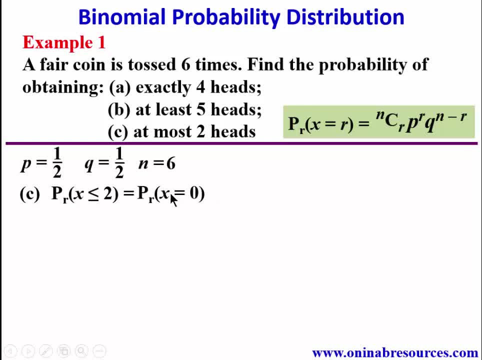 to give us probability of getting 0, that is, X is equal to 0 or probability of X is equal to 1, one or probability of x is equal to two. so we now find the probability of x is equal to zero, that of x is equal to one and x is equal to two. and sum them up so that probability of x is equal. 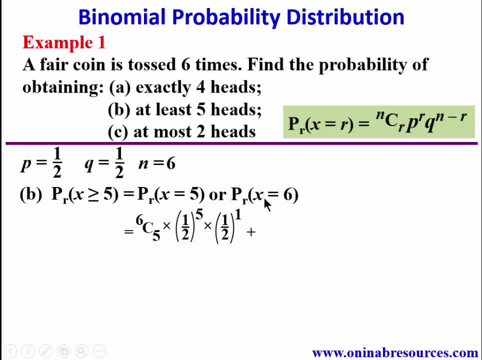 which means plus for probability of success is equal to six. we have it as six combination six times p, which is one over two raised to power six, then times failure, which is one over six raised to power zero. so six combination five gives six times one over 32 times one over two, plus six combination six. 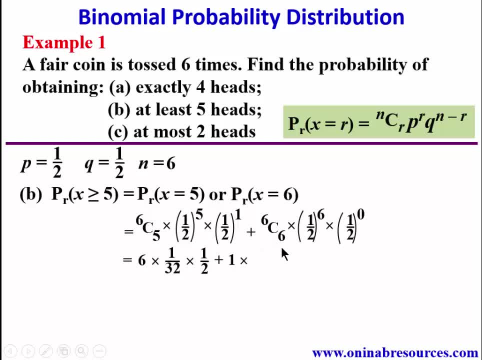 is one times one over 64 times one, since half raised to power zero is one. so simplifying this, we have it as 6 over 64 plus 1 over 64, and that gives our final answer as 7 over 64, which is the probability of obtaining at least five heads when a coin. 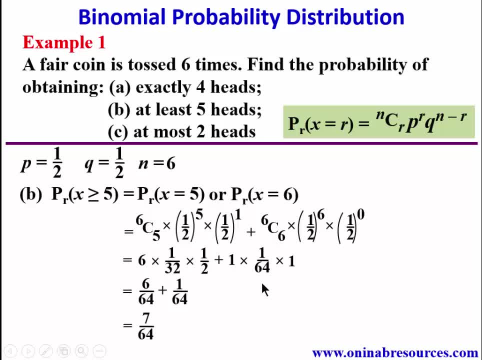 is tossed six times. so we go to see part of the problem. for c, at most two, at most the highest we can get there two heads. so in this case now we are going to have it as p of x less than or equal to two, which is going to give us probability of getting zero. that is, x is equal to zero or 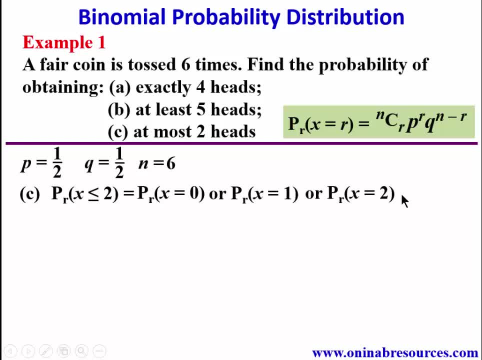 probability of x is equal to one or probability of x is equal to two. so we now find the probability of x is equal to zero, that of x is equal to one and x is equal to two. and sum them up so that probability of x is equal to zero, now will be six combination, zero times p, which is half raised to. 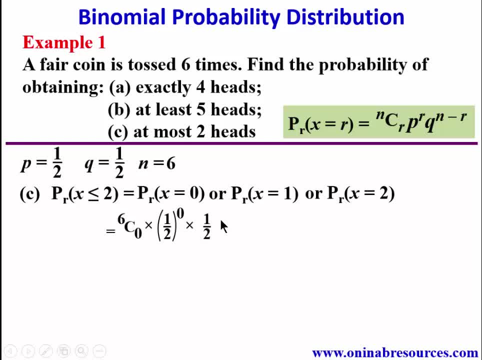 power zero times q, which is half raised to power six. then plus p, which is half raised to power six, then plus, probability of x is equal to one, will be six combination: one times p raised to power one, which is half raised to power one times half raised to power five. remember, when you add the powers, 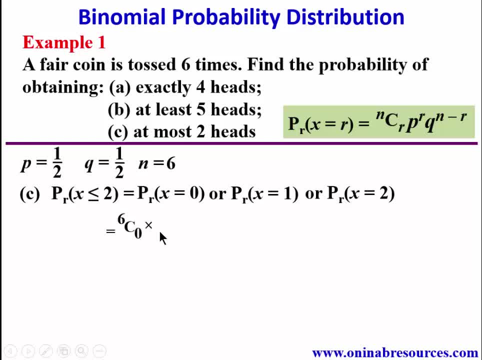 to zero. now will be six combination: zero times p, which is half raised to power, zero times q, which is half raised to power. six then, plus probability of x is equal to one, will be six combination: one times p raised to power. one, which is half raised to power, one times half raised to power. five. 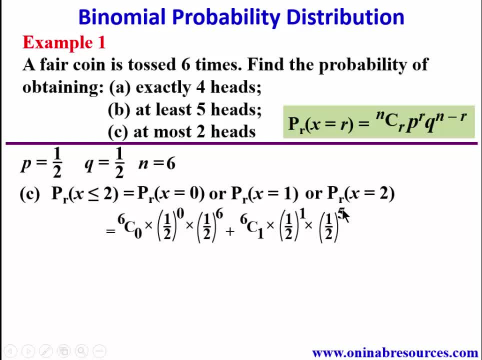 remember, when you add the powers here you are meant to have six, which gives the total number of n, then plus probability of x is equal to zero- will be six combination two times one over two, squared times one over two, to the power of four. and simplifying this six combination zero is one times one, times one over sixty four, then plus. 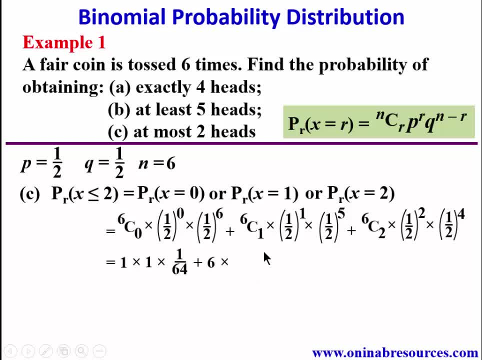 six. combination one gives six times half times one over thirty two. then also plus six. combination two gives fifteen times one over four times one over sixteen. so this is simplified as one over sixty four plus six over sixty four, then plus fifteen over sixty four. simplifying finally, we have one plus six. 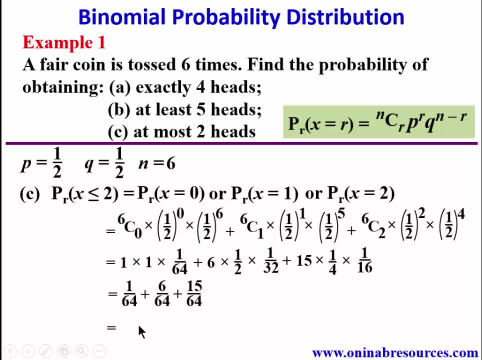 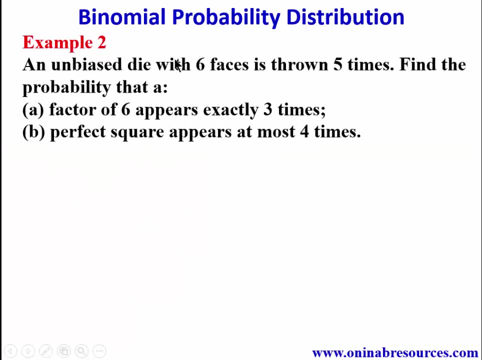 which is seven plus fifteen. twenty two over sixty four, and in the simplest form we have it as eleven over thirty two, and that gives the probability of getting at most two heads when a coin is tossed six times. so we go to example two, i'mton's two, an um biask die with six faces is thrown five times. 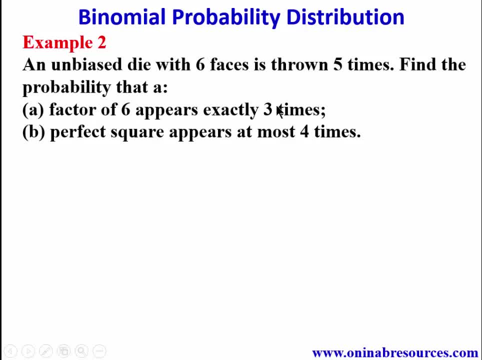 find the probability that a, a factor of six, appears exactly three times b. a perfect square, appears at most four times. in this problem we are going to treat a and b separately because the event in a is different from the event in b, so, starting from a, we need: 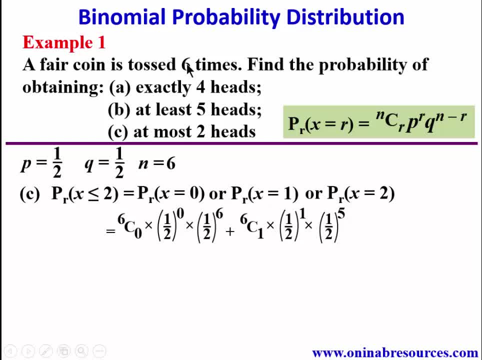 here you are meant to have six, which gives the total number of n. then plus probability of x is equal to two, will be six combination, two times one over two, squared times one over two, to the power of four. and simplifying this six combination, zero is one times one times one over 64. then plus six combination, one gives six times. 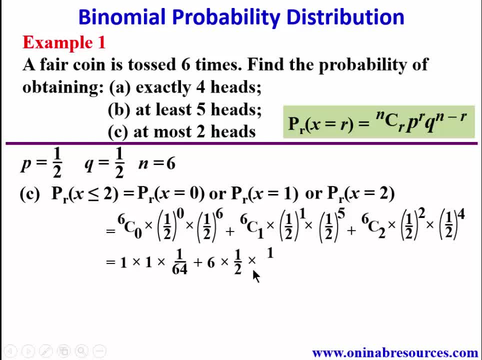 half times one over 32, then plus four times one over, six times one over, two times one over. also plus 6, combination 2 gives 15 times 1 over 4 times 1 over 16. so this is simplified as 1 over 64 plus 6 over 64, then plus 15 over 64. simplifying finally. 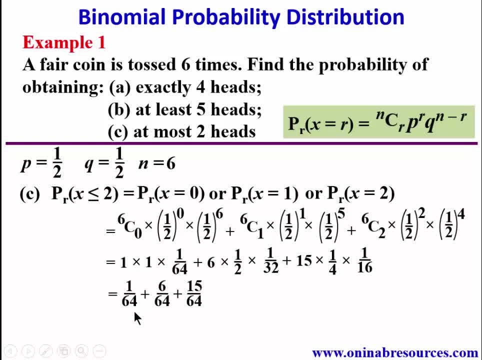 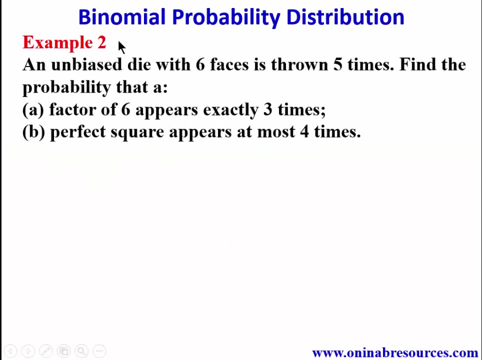 we have 1 plus 6, which is 7 plus 15, 22 over 64, and in the simplest form we have it as 11 over 32, and that gives the probability of getting at most 2 heads when a coin is tossed six times. so go to example 2. example 2: an unbiased die with. 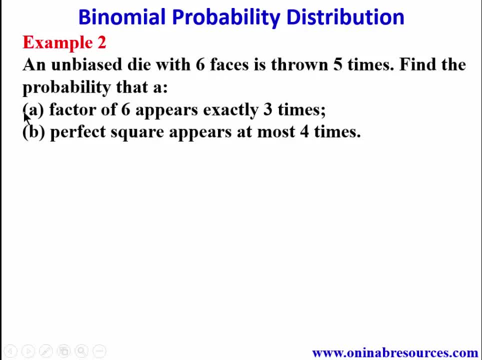 six faces is thrown 5 times. find the probability of getting the coin throw it's thrown five times. find the probability of getting the coin throw it's thrown five times. find the probability that a- a factor of six, appears exactly three times. b- a perfect square, appears at most. 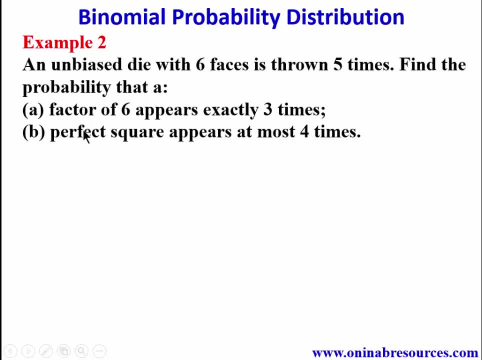 four times in this problem. we are going to treat a and b separately because the event in a is different from the event in b. so, starting from a, we need to get our sample space, which is the place on the faces of a fair die. so we have it as 1, 2, 6 and n of s is 6, the event space of getting a. 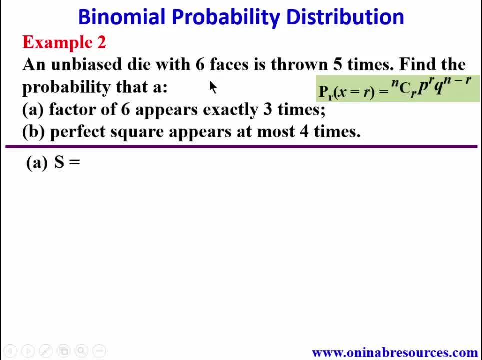 to get our sample space, which is the numbers on the faces of a fair die. so we have it as one to six and n of s is six. the event space of getting a factor of six is f and the factor of six here are one, two, three and six, and n of f is equal to four. the essence: 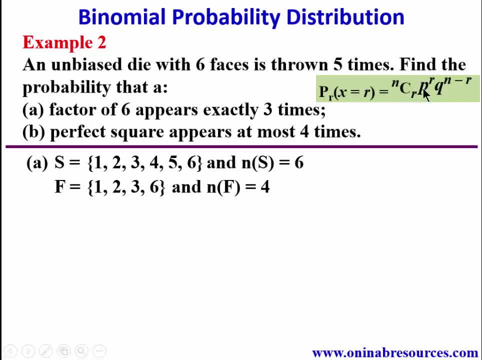 of having these is to enable us get the values of p and q. so to get our q, which is the probability of success for obtaining a factor of six, will now be four over six. in the simplest form we have it as two over three. then the probability of not having a factor of six, which is q, 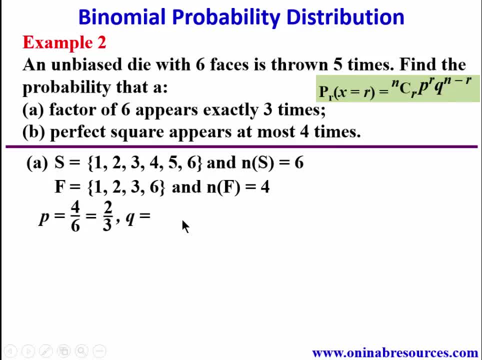 will be one minus two over three, and that gives one over three. our n here is five, since the die is shown five times, and our r, which is exactly three times, will give us three, so that probability of x is equal to three will be five combination three times two over. 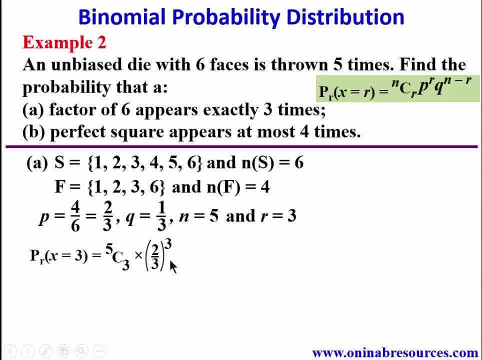 three raised to power three times one over three raised to power two, since two plus three gives a five, which is our n. so five combination three gives ten times. simplifying this, that will give us eight over twenty, seven times one over nine, and finally we have it as: 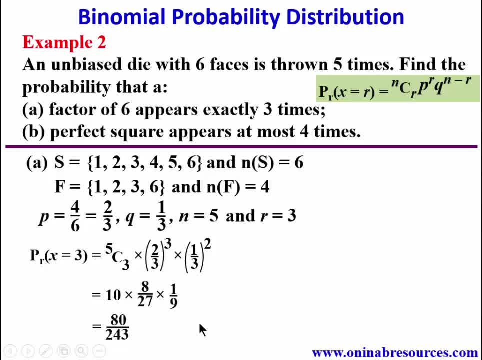 80 over 243, and that is the a part of example two. we're going to be part of the problem here. we still maintain our sample space, which is still one to six, and n of s is six. therefore, perfect square. we represent the event space as e, which is going to give us a 1. 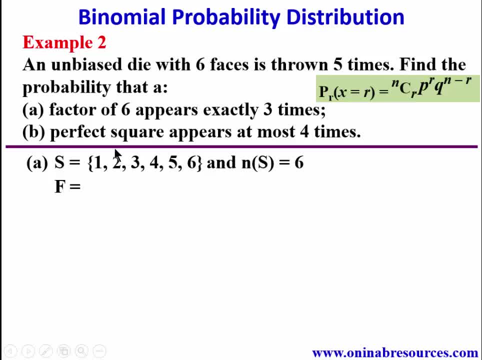 factor of 6 is F and the factor of 6. here are 1, 2, 3 and 6, and N of f is equal to 4. the essence of having this is to enable us getting the value of p and q, so to get our q, which is the probability of success for obtaining a factor of. 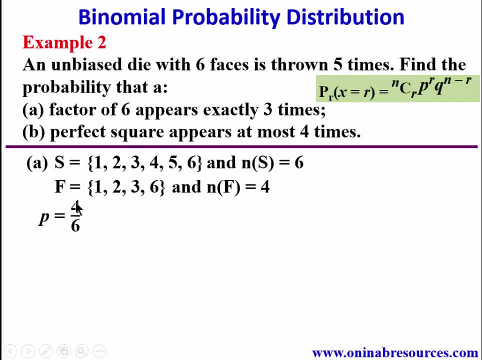 6 will now be 4 over 6.. in the simplest form we have it as 2 over 3. then the probability of not having a factor of 6, which is q, will be 1 minus 2 over 3, and that gives 1 over 3.. our n here is 5. 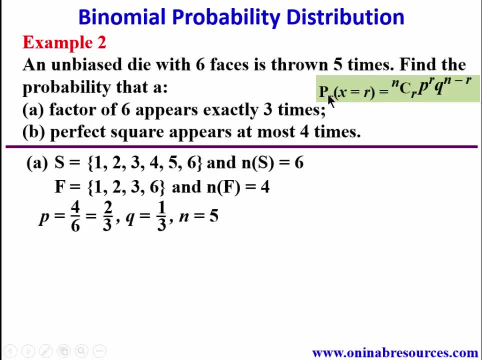 since the die is shown five times, and our r, which is exactly three times, will give us three, so that the probability of x is equal to three, will be five. combination: three times two over three. raised to power three times one over three. raised to power: two since two. 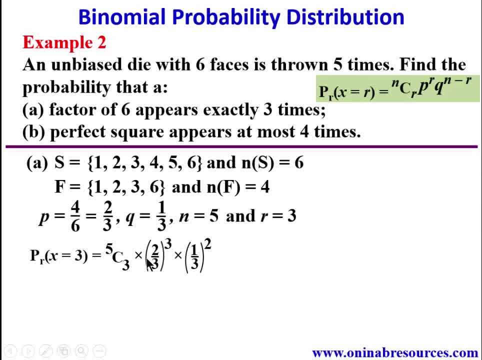 plus three gives a five, which is our n, so five combination three gives ten times. simplifying this, that will give us eight over twenty, seven times one over nine, and finally we have it as 80 over 243. and that is the a part of example two. 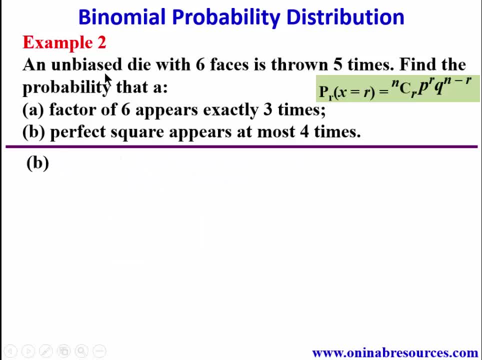 we're going to be part of the problem. um, here we still maintain our sample space, which is still one to six, and n of s is six. then, for perfect square, we represent the event space as e, which is going to give us a 1 comma four. the perfect squares here are one and four and we have n of e to be equal to two. this 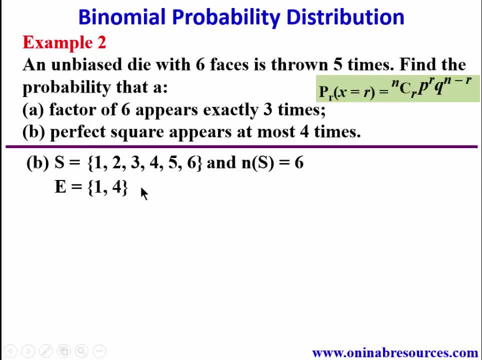 the perfect squares here are one and four and we have n of e to be equal to two. this will enable us get the values of p and q, so probability of having success, that is, having a perfect square, will be two over six, which is equal to one over three, and for q, which is the probability. 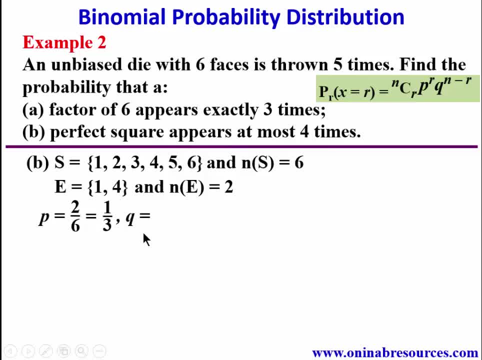 of not having a perfect square would be 1 minus 1 over 3, which is 2 over 3, and our n is still 5, and then our r. since it is at most four times, then the highest we can get there is four, which means we can have it as a zero: one, two, three and four. we can't get more than four since. 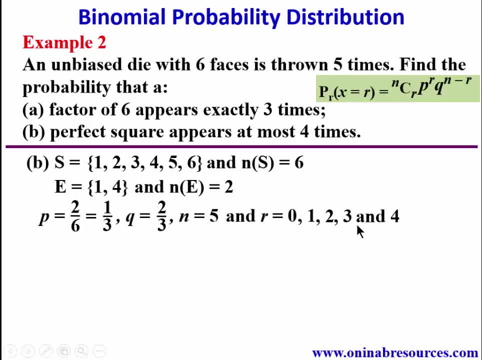 it is at most four times. so the probability now of having x less than or equal to 4 will be probability of 1 minus. probability of x is equal to 5 because in the entire space it is only 5. since it is true 5 times, it is only 5 that is not there. so we can just quickly say 1 minus. 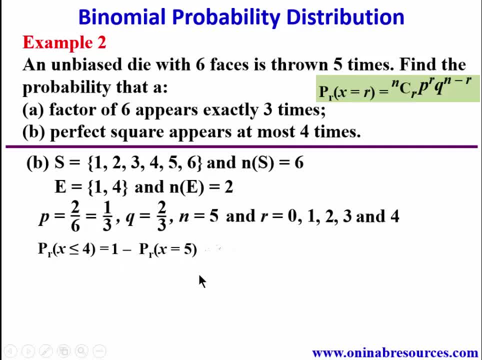 probability of getting 5. so that's going to give us 1 minus 5 combination, 5 times p, which is 1 over 3 to the power of 5 times 2 over 3 to the power of 0, and that will give us 1 minus 5 combination. 5 is 1. 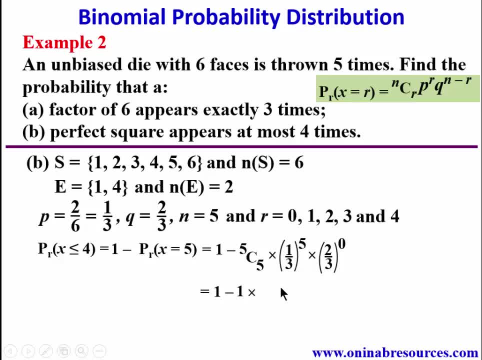 1 over 3 to the power of 5 is 1 over 243. then times 1, since 2 over 3 to the power of 0 is 1, so that 1 minus 1 over 243 will give us 242 over. 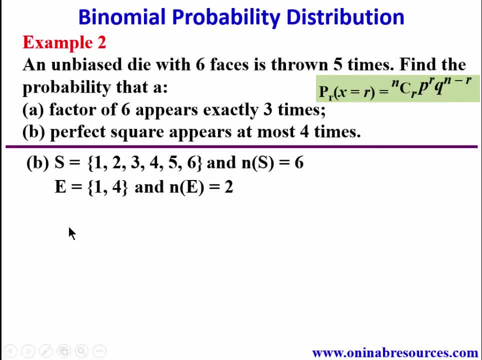 we enable us get the values of p and q, so probability of having success, that is, having a perfect square, will be two of us is, which is equal to one over three, and for q, the probability of not having a perfect square will be one minus one over three, which is two. 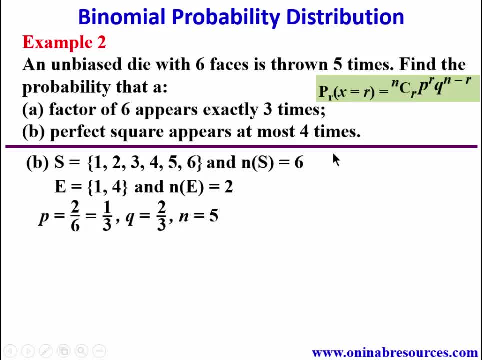 over three and our n is still five, and then our r, since it is at most four times, then the highest we can get there is four, which means we can have it as a zero one, two, three and four. we can't get more than four, since it is at most four times. so the probability now of having x less than or equal, 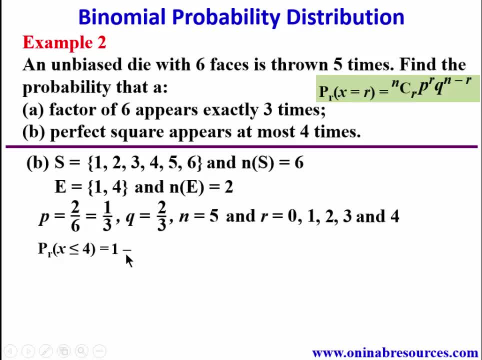 to four will be probability of one minus probability of x is equal to five, because in the entire space it is only five. since it is thrown five times, it is only five. that is not there. so we can just quickly say one minus probability of getting five. so that's going to give us one minus five, combination five: 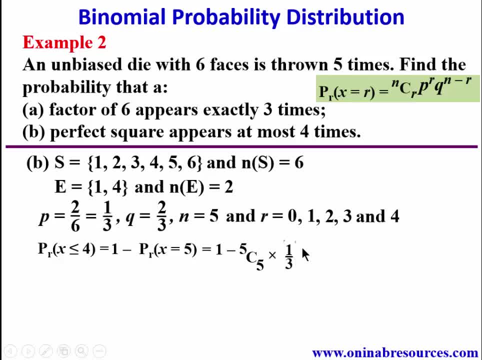 times p, which is one over three to the power of five, times two over three to the power of zero, and that will give us one minus five combination: five is one. one over three to the power of five is one over two hundred and forty. three, then, times one, since two over three to the power of zero is one, so that one 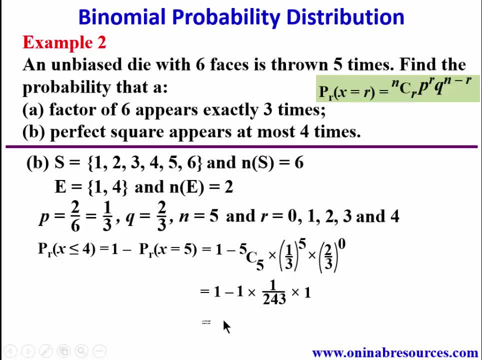 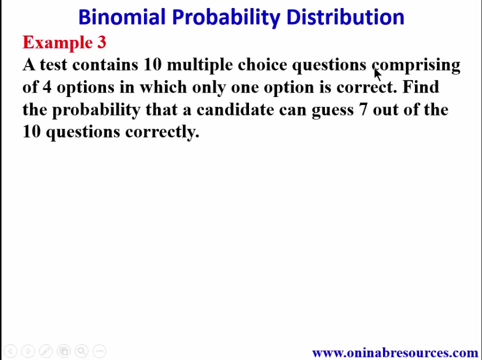 minus one over 243, we give us 242 over 243 and that is the probability of obtaining perfect square at most four times from throwing a die for five times. and that's all for example two. so we go to example three. example three: a test contains ten multiple choice questions comprising of four. 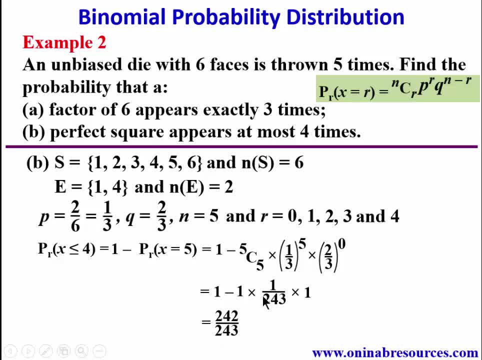 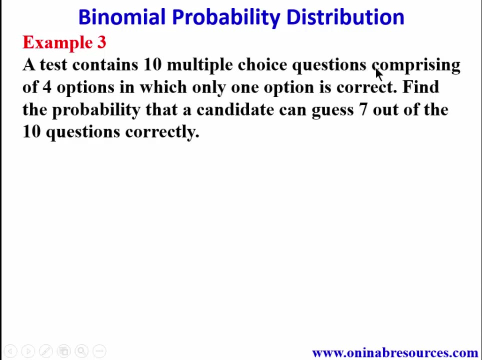 243, and that is the probability of obtaining perfect square at most four times from throwing a die for five times. and that's all for example two. so we go to example three. example three: a test contains ten multiple choice questions comprising of four options in which only one option is correct. find the. 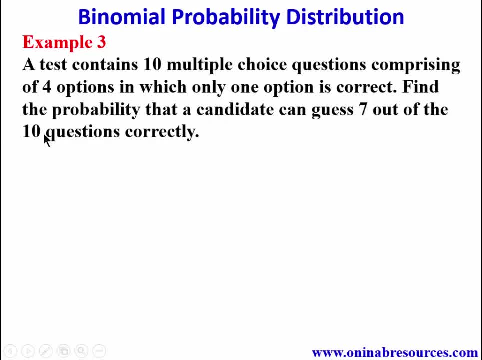 probability that a candidate can get seven out of the ten questions correctly. the probability of getting it correctly is only one over four. we get that and okay, let's go. the probability of getting one of the questions correctly is one over four and the probability of getting it wrong is three over four, so that 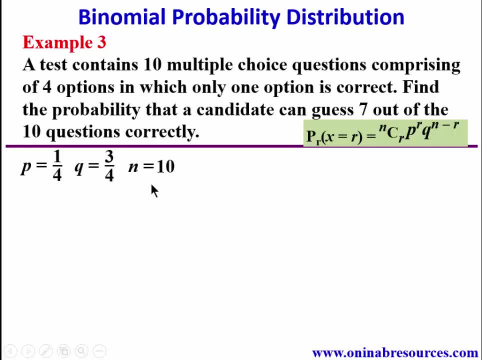 our end is ten. since there are ten multiple choice questions and our r is going to be seven, so that the probability of x is equal to 7, will be 10. combination 7 times 1 over 4 to the power of 7 times 3 over 4 to the 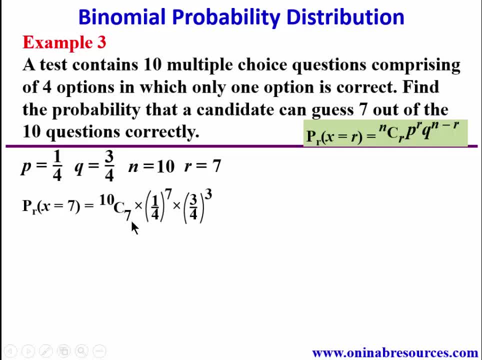 power of 3, so 10. combination 7 is 120 times 1 over 16. 384. that is, 4 is to power 7 times 27 over 64. so, simplifying this, we have our answer as 0.0030899. 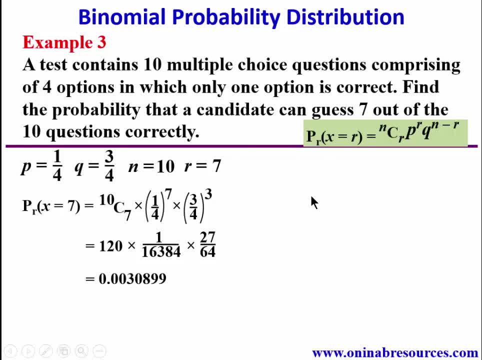 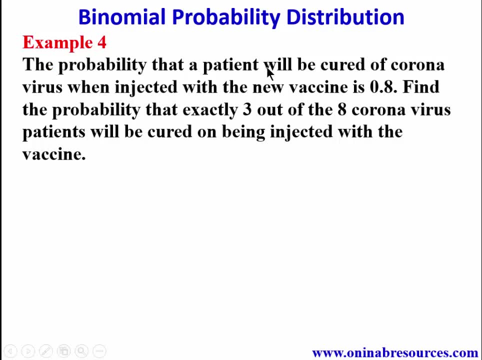 which represents the probability that a student can guess seven out of the ten questions correctly. and at the end of example three we go to example four. for example four, the probability that a patient will be cured of corona virus when injected with the new vaccine is 0.8. 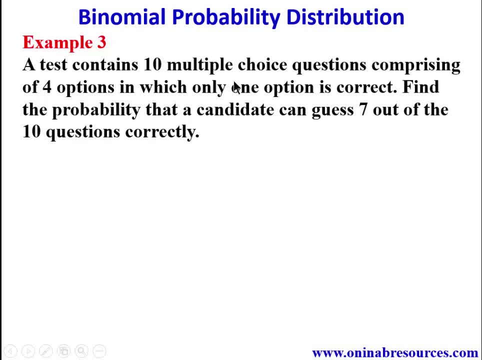 options in which only one option is correct. find the probability that a candidate can get seven out of the ten questions correctly. the probability of getting it correctly is only one over four. we get that and okay, let's go. the probability of getting one of the questions correctly is one over four. 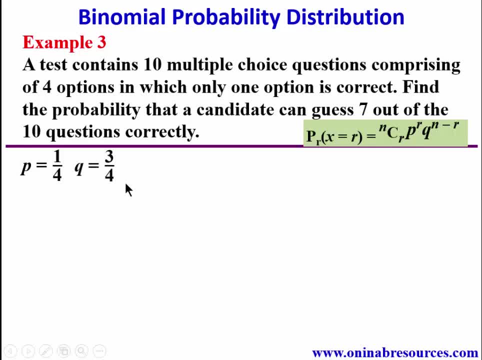 and the probability of getting it wrong is three over four, so that our n is ten. since there are ten possible choice questions, and our r is going to be seven, so that the probability of x is equal to seven, will be ten. combination seven times one over four, to the power of seven times three over four. 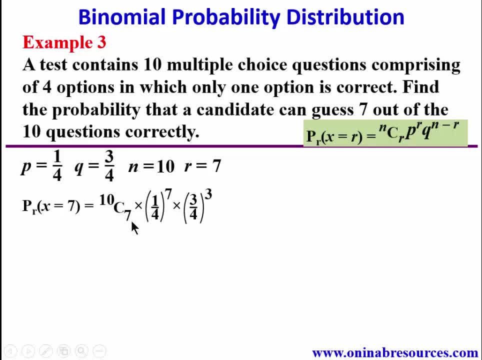 to the power of three. so ten combination seven is one hundred and twenty five times one over sixteen thousand three hundred and eighty four, that is, four is to power seven times 27 over 64. so, simplifying this, we have our answer as 0.0, which represents the probability that a student can guess seven out of the. 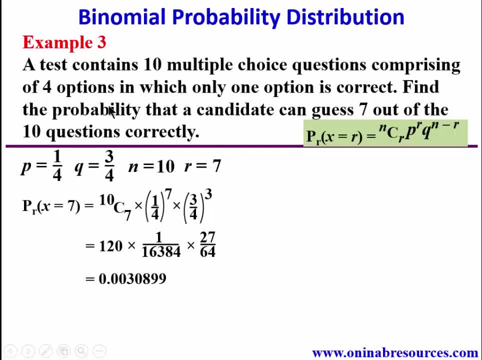 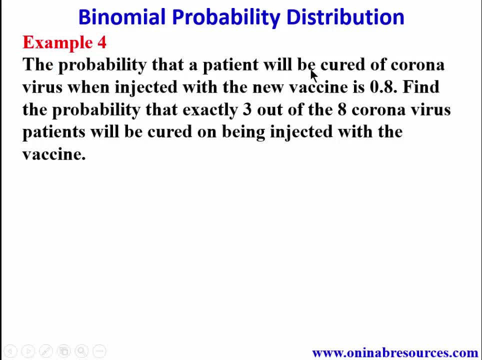 ten questions correctly, and at the end of example three we go to example four. for example, for the probability that a patient will be cured of corona virus when injected with new vaccine is 0.8, finding probability that exactly three out of the age corona virus patients will be cured on being injected with the. 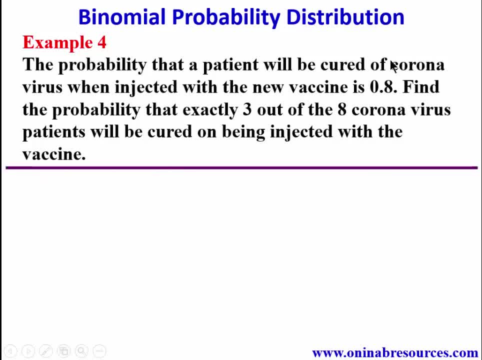 vaccine. so again we know our probability of success, that is, P is 0.8 and Q will be 1 minus 0.8, which is 0.2. our end is equal to its, since there are its patients, and our expectation is 3.